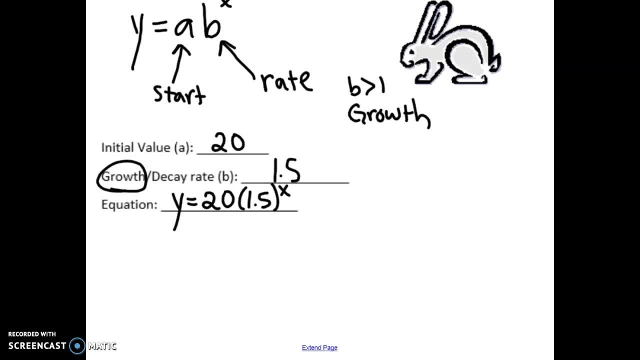 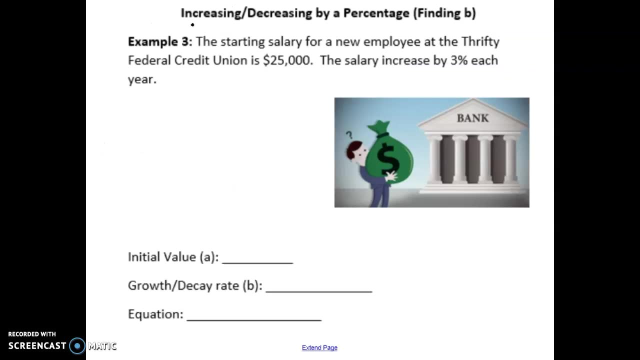 Don't forget that x power guys, because this is an exponential function, It does need to have that exponent. Now, that seemed pretty easy because the two values, 20 and 1.5, We're directly in the word problem already. but we do have problems like this one where we are increasing or decreasing by a. 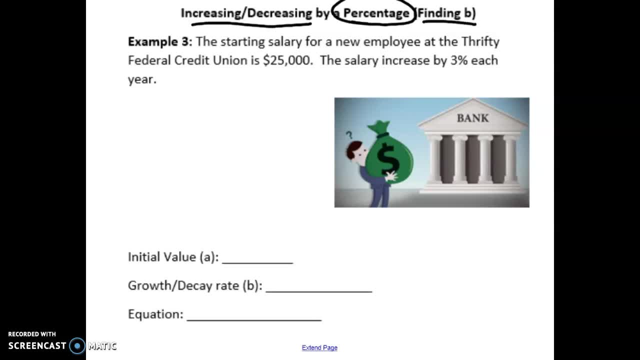 Percentage and we have to find out what B is. we don't know B right off the bat, so let's read through the problem first. The starting salary for a new employee at the Thrifty Federal Credit Union is $25,000.. That's his starting salary, So that should tell you right off the 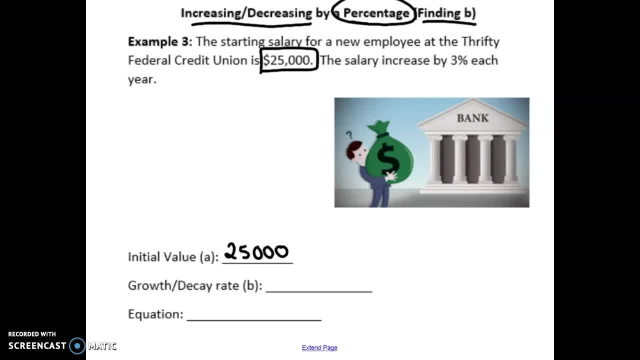 bat. that is our A value. The salary increases by 3% each year. So, in order to find out what our B value is, we know that we're increasing by 300%. If you see the word increase, that means we're going to be adding. We're going to take 100%, because we always start with 100%, 100% of this. 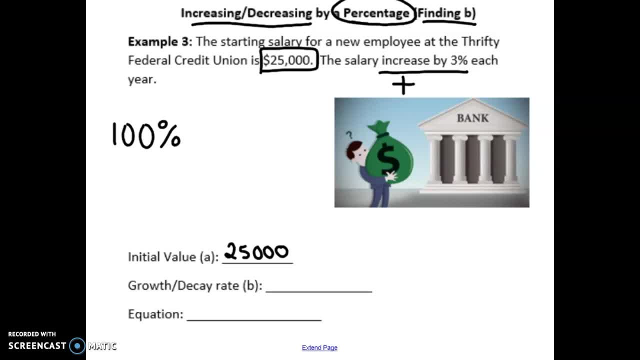 salary: 100% of anything. Whatever you are given initially, you have 100% of it And if we're increasing, we add, and we're adding, in this case, 3%. Keep in mind that if this had been decreasing, 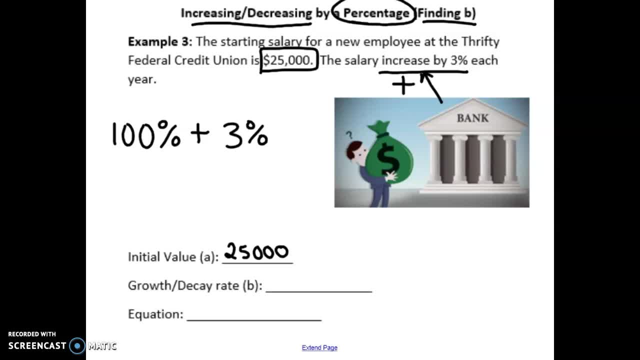 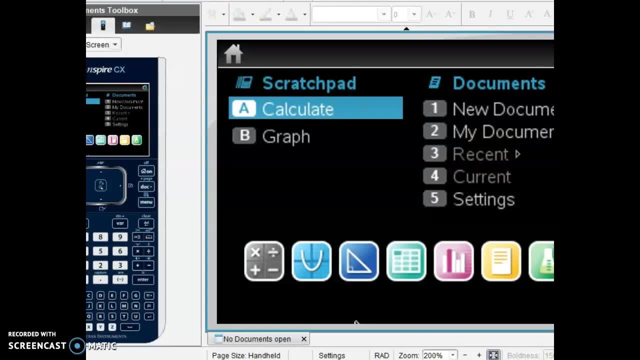 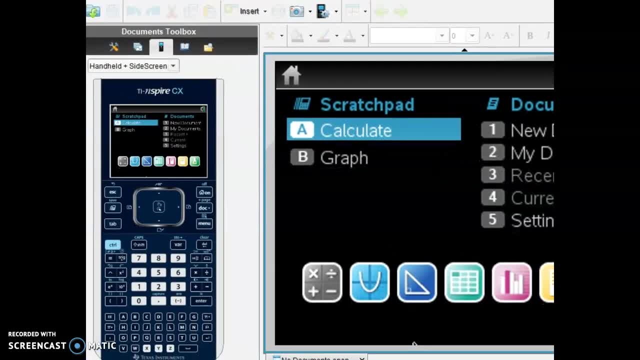 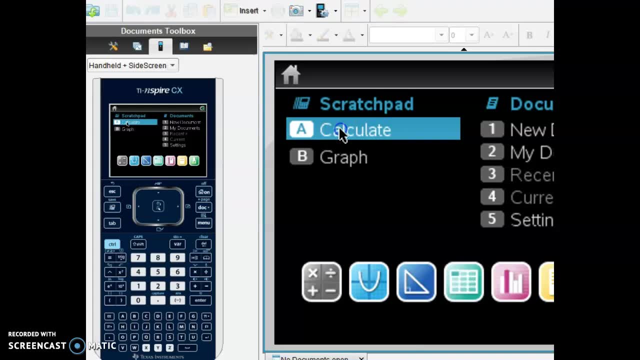 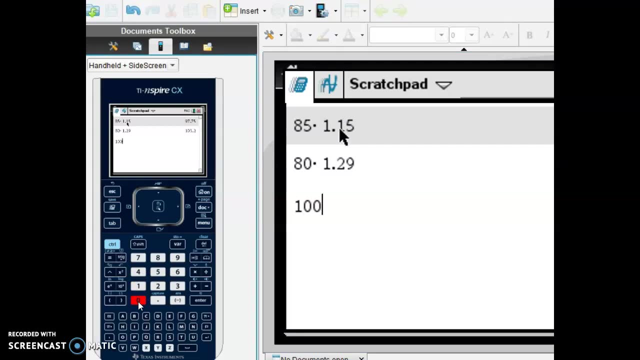 make it that much smaller. I guess I will just move it down here so we can see it a little bit better. Okay, so on the calculator. what you would do is you would go to calculate and you would type in 100% plus 3%, So 100,. go to the question mark down here below the enter button and choose. 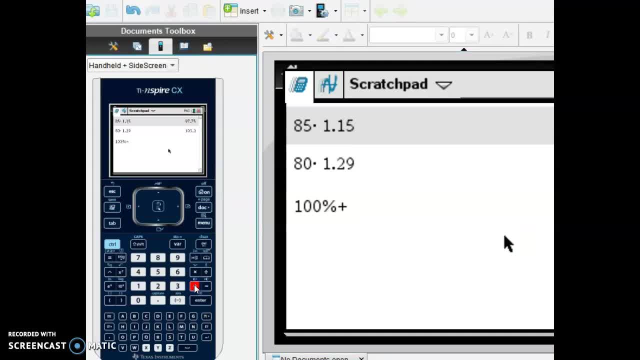 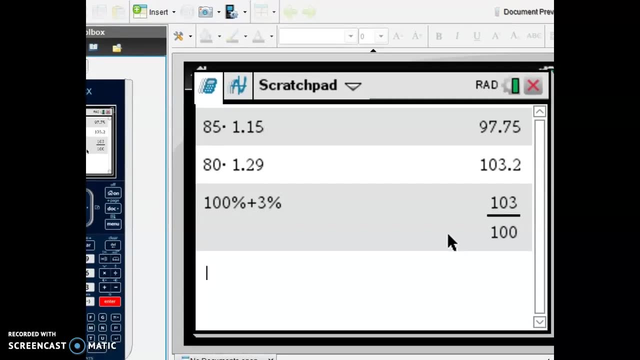 progress percent. we're adding 3%, so I need to find the percent button again and then we hit enter and we will get our B value. in this case, our B value is- you can see it over here: it gives us a fraction. so instead of hitting enter, hitting.